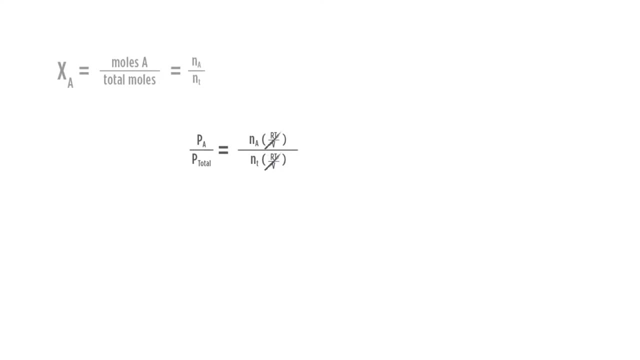 here. RT over V. RT then cancels giving us NA over NT, And we know that A over NT is the mole fraction for A. So therefore PA over PT is related to XA. We can then convert that into the formula. 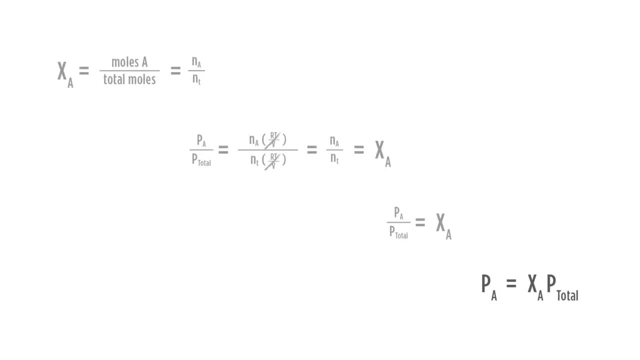 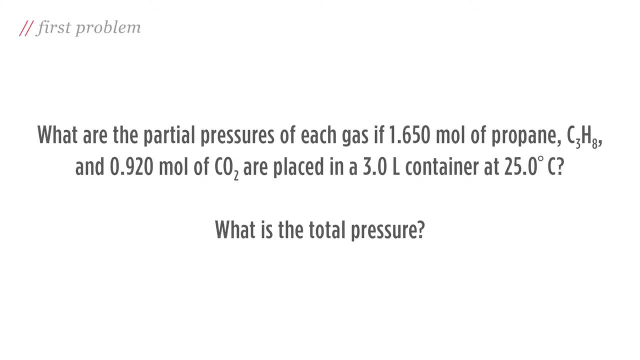 PA equals mole fraction A times the pressure for the total. Okay, let's use these two expressions Here. we have two different problems for the mole fraction. First problem: what is the partial pressure of each gas if 1.65 moles of propane, C3H8, and 0.920 moles of carbon dioxide are placed? 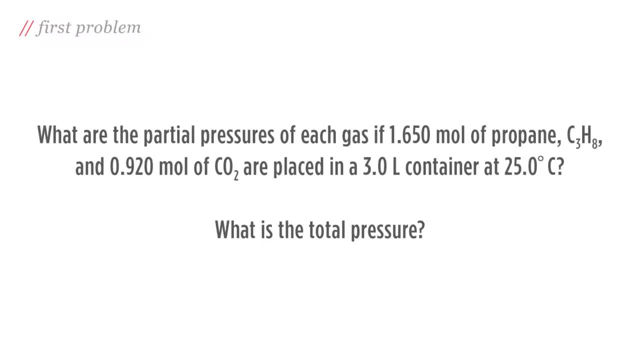 in a 30 liter container at 25 degrees Celsius, What is the total pressure? So, if we analyze the question here, it's giving us some information, but it's actually asking us to calculate the things. One: we're going to need the partial pressures for each: the propane. 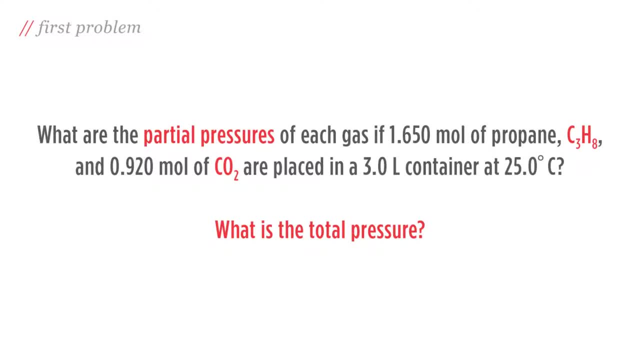 and the CO2.. And it has a second question: what is the total pressure? So we're also going to have to calculate the total pressure. We know that it gives us a number of moles of propane and CO2 and it gives us the volume and the 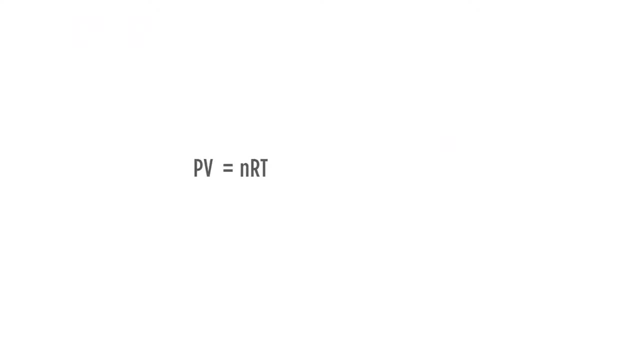 temperature. We can calculate the pressure by using pv equals nRT. If we convert pv equals nRT to get pressure by itself, we'll see that we get nRT over V For partial pressure for propane. we just need to plug in our values So. 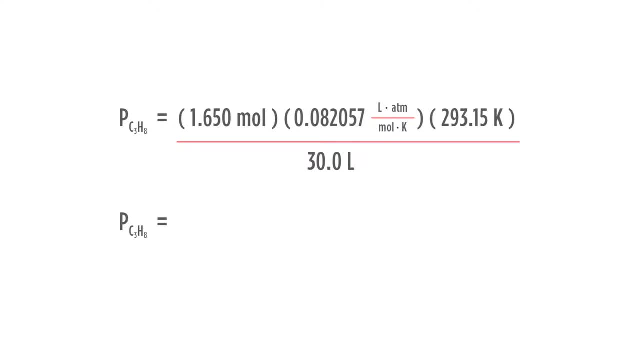 1.650 moles times the constant R, times 293.15 Kelvin, which is the conversion of 25 degrees Celsius to Kelvin divided by 30.0 liters. We do that calculation, we look at our calculation, we look at our. 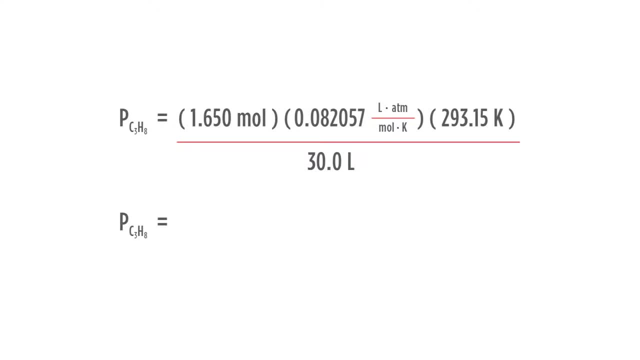 significant figures and we see that our answer here is going to be: partial pressure of propane is equal to 1.32 atmospheres. We can do the same calculation using p equals nRT over V for the partial pressure of CO2.. Here we 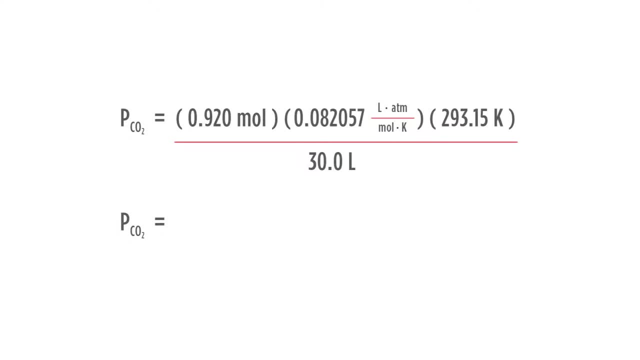 have partial pressure of CO2, plug in our values: 0.920 moles times the constant R times 293.15 Kelvin, which is the conversion of 25 degrees Celsius divided by 30.0 liters, That gives us a partial pressure of CO2 of 0.738 atmospheres. 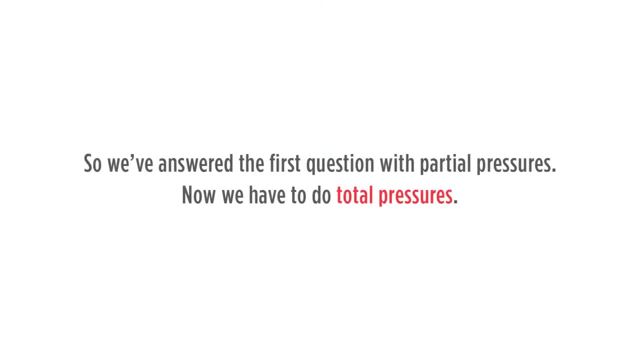 So we've answered the first question, the partial pressures. Now we have to do total pressures. Remember, there's two ways to do this. One way we can look at: partial total is equal to the partial pressures of propane plus the partial pressure of CO2.. 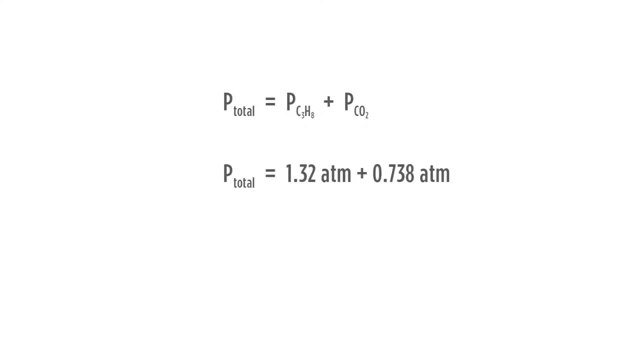 We already calculated these, so we just have to plug them in. So the total pressure is 0.738 atmospheres. Add those together- remember our significant figures- and we come out with the total pressure equals 2.06 atmospheres. At this point we've 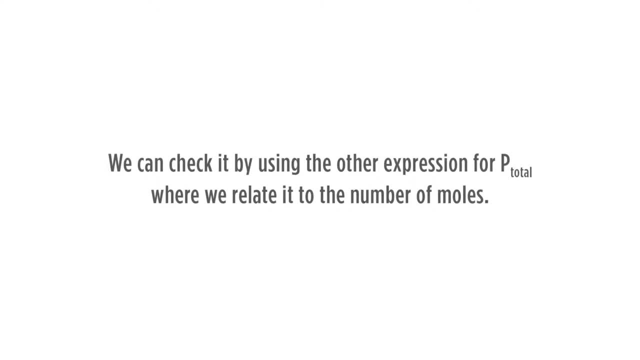 answered our problem, but we can check it by using the other expression for pressure, total, where we related to the number of moles. So we can take the values directly out of the question: 1.650 moles plus the number of moles. for. 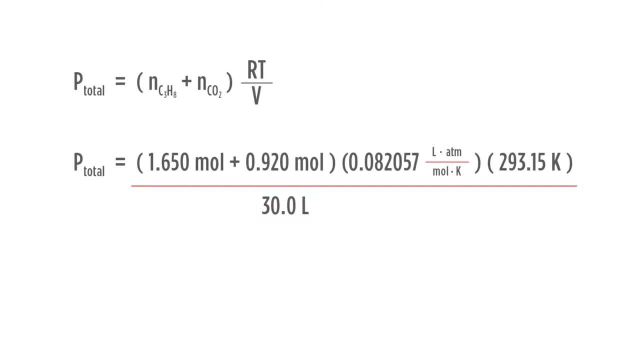 CO2, 0.920 moles. So we can take the values directly out of the question, 1.650 moles plus the number of moles for CO2, 0.920 moles, and we can put that in the formula. 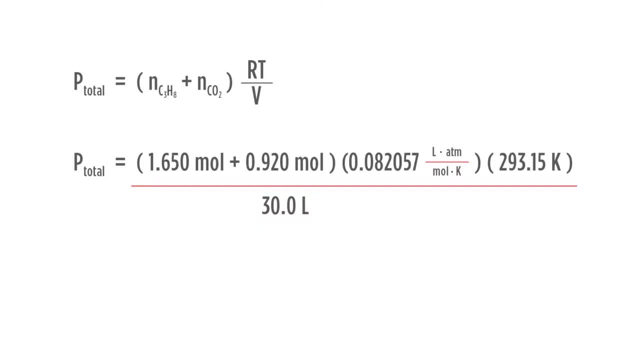 number of moles of propane plus number of moles of CO2 times RT over V. We plug all those values in, We do our calculation again following significant figures, and we come up with the pressure total of 2.06 atmospheres. Now let's look at calculating the ratio. 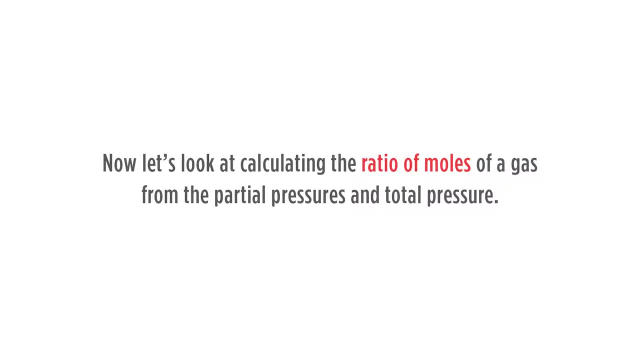 of moles of a gas from the partial pressures and total pressure For that value. we're going to look at this problem. What is the mole fraction of CO2 in a mixed mixture of gases with a partial pressure of CO2 of 1.75 atmospheres and of nitrogen? 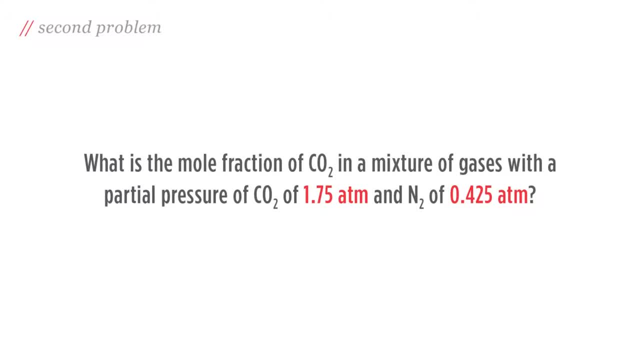 of 0.425 atmospheres. So in this case we're given the partial pressures. So we can remember that the mole fraction of CO2, which is what the question is asking for- is going to be the partial pressure of CO2 over the total pressure. We have the partial pressures of. 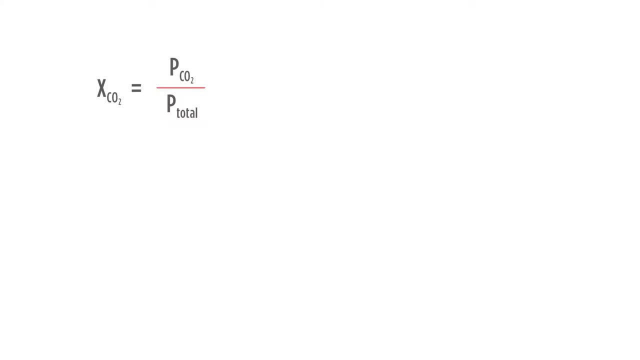 both CO2 and nitrogen, But not the total pressure. We can calculate the total pressure by adding the two partial pressures. So P total equals partial pressure of CO2 plus the partial pressure of nitrogen. We can look those values up. Partial pressure of CO2 is 1.75 atmospheres from the question. 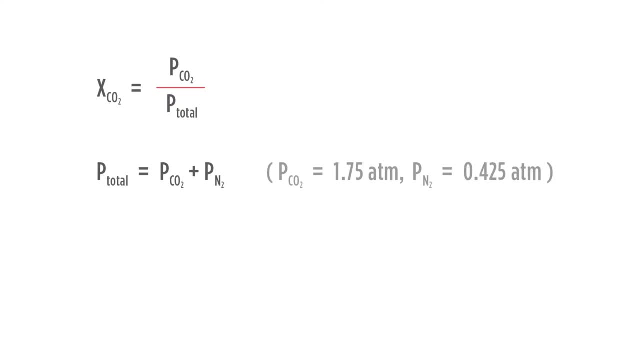 Partial pressures of nitrogen is 0.425 atmospheres from the question. We put those into the formula, add those together and we get a total pressure of 2.18 atmospheres. Now we have both the values. we need to calculate the mole fraction. So we take the mole fraction. 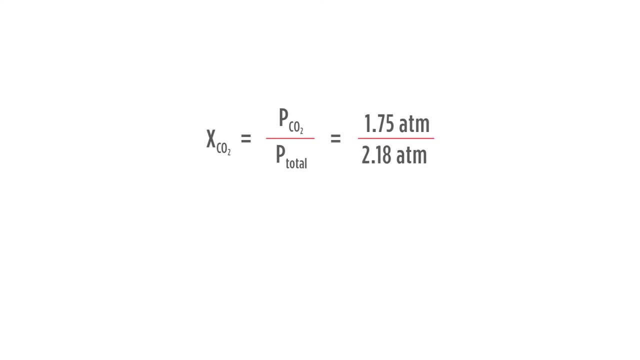 as the partial pressure of CO2 over the total pressure. so 1.75 atmospheres over 2.18 atmospheres. Do our calculation and we come up with the mole fraction of CO2 of 0.80.. Notice in this: 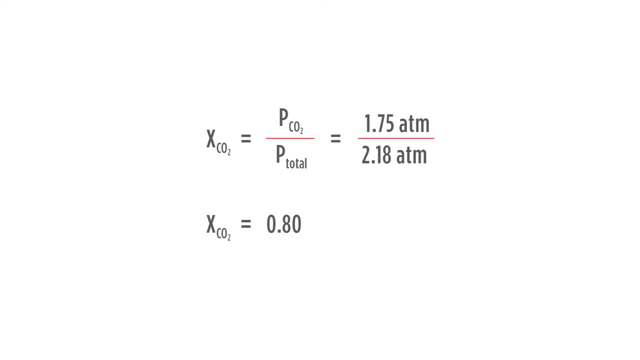 case that we do not have any units, because partial pressure of CO2 is in atmospheres and the total pressure in atmospheres, So those cancel, leaving us with a unitless molecule quantity. Practice: partial pressures: calculating total pressure and mole. 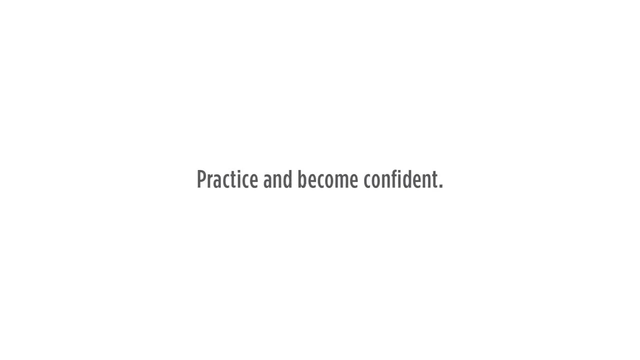 fractions, Practice and become confident. 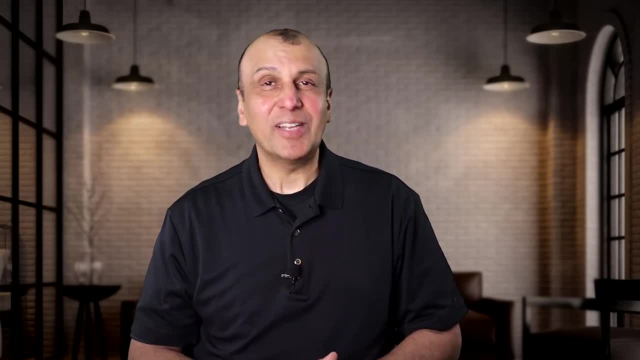 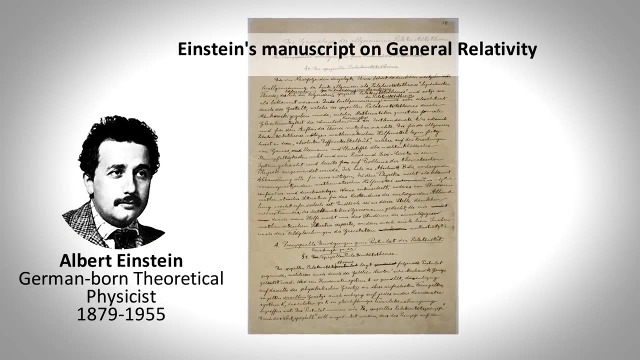 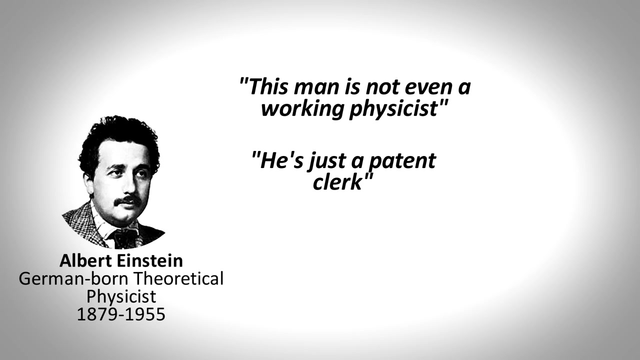 When Einstein first published the special theory of relativity in 1905, he was either vehemently ridiculed or ignored. People thought it was just too weird and radical to be real. This guy is not even a working scientist, He's just a patent clerk, some said. How dare he challenge the greatest? 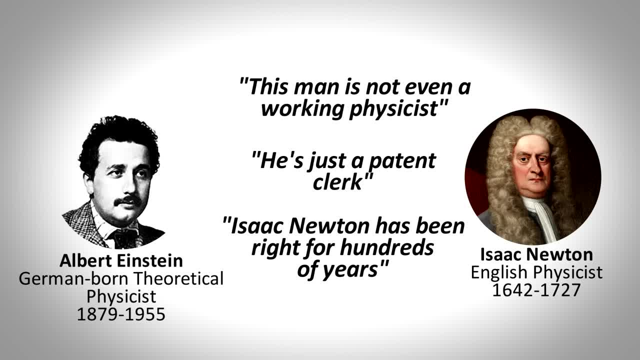 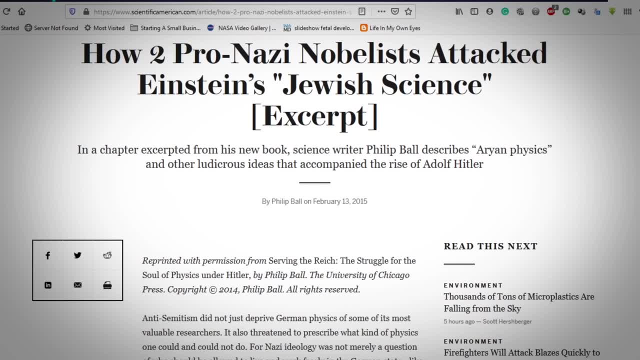 scientist that ever lived, Isaac Newton, whose theories have been proven to be correct for hundreds of years. Some politicians even insulted his religious heritage and called it Jewish science, a way to subvert traditional culture and thinking. How did Einstein feel about this? Well, 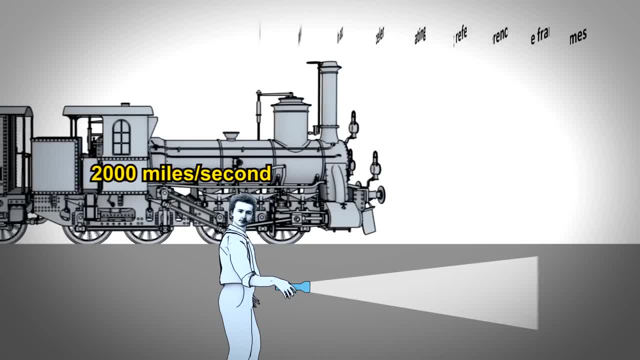 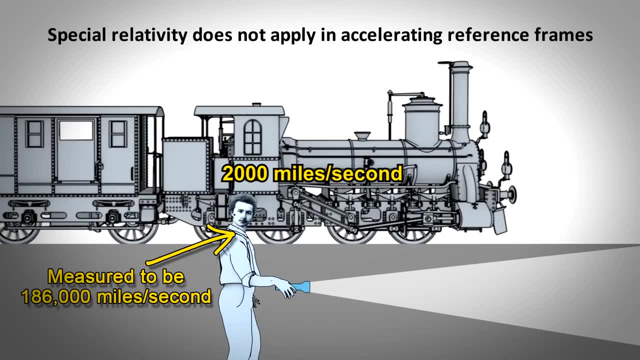 he wasn't satisfied with this theory either. He was unhappy because the theory only applied to observers moving in a straight line at a constant speed. The theory did not apply if gravity was present or if the observer was accelerating. Einstein was known, however.